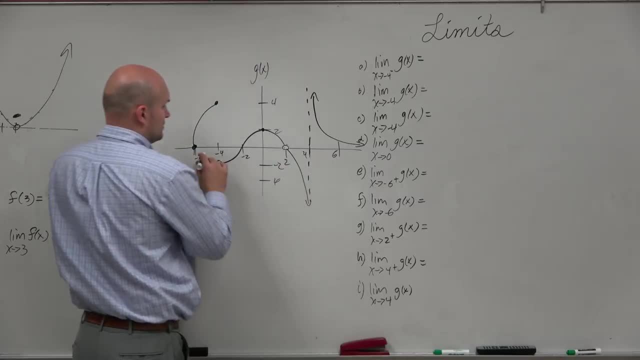 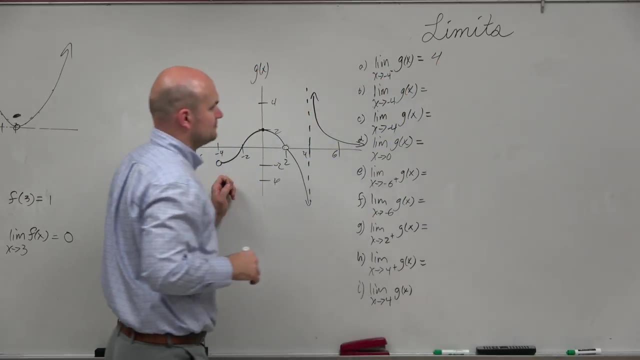 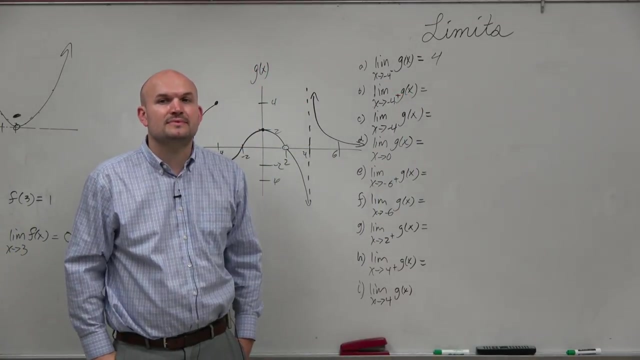 value 4.. You're approaching 4, right. So we could say the limit as x approaches negative 4, from the left is equal to 4.. Oh, I didn't see that. Yes, OK, so you have all the arrows going from x to the right. 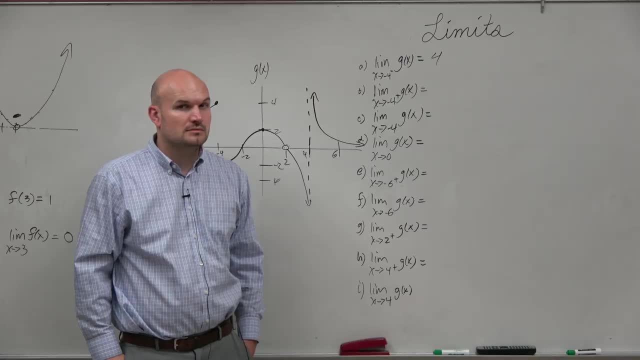 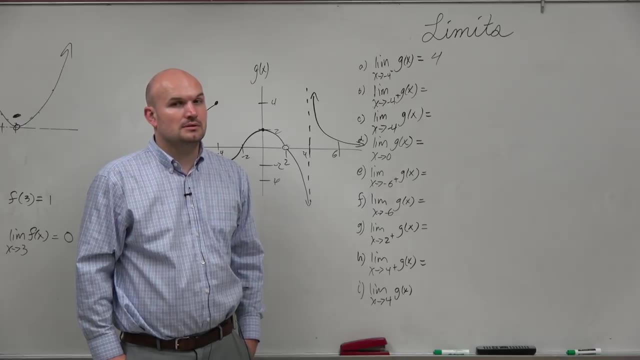 Could you ever write it like: for our sake, could you ever write x on one side, going to the left and then the right? So if you're approaching x, Yeah, I mean I can say that makes sense, but that's not like you're saying. 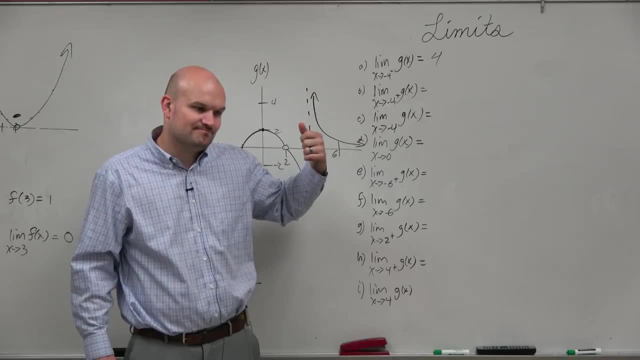 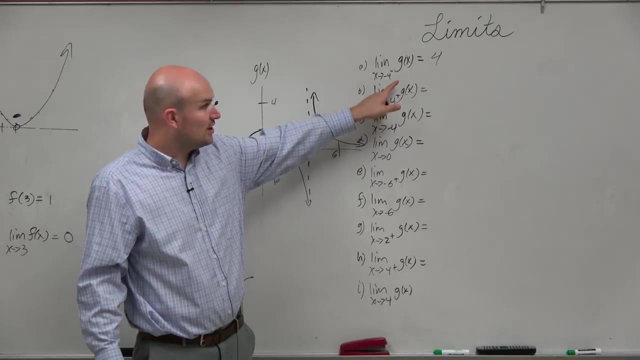 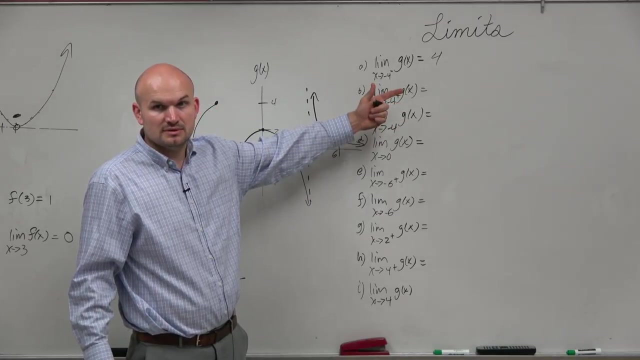 That's not your standard notation, So people probably wouldn't know what you mean by that. So we just write it and read it as: x approaches negative 4.. And the reason why the left is like: from the left, x approaches negative 4 from the right. 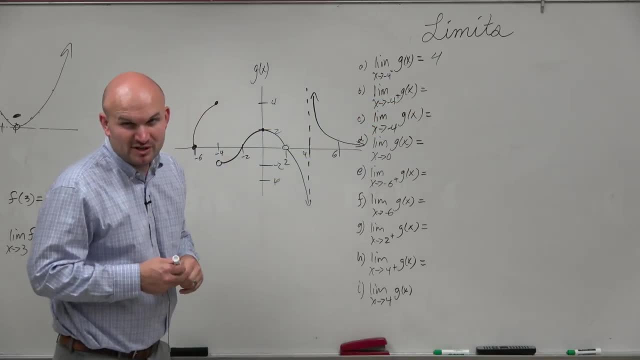 That little plus just means from the right hand side. So yeah, I would avoid just doing something that's not at least to your standard notation. So now let's go and take a look. What about, as we approach, negative 4 from the right? 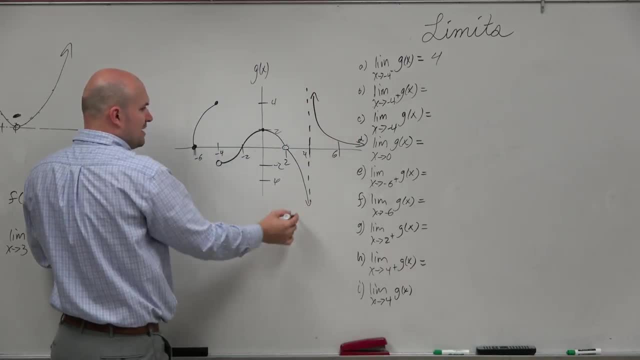 So we look at our graph, We kind of take out our right hand. We say, all right, let's follow this graph from the right. As we approach from the right, we get really, really close to which y value Negative 2.. 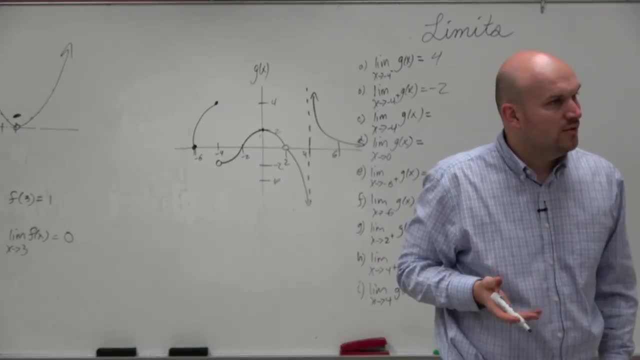 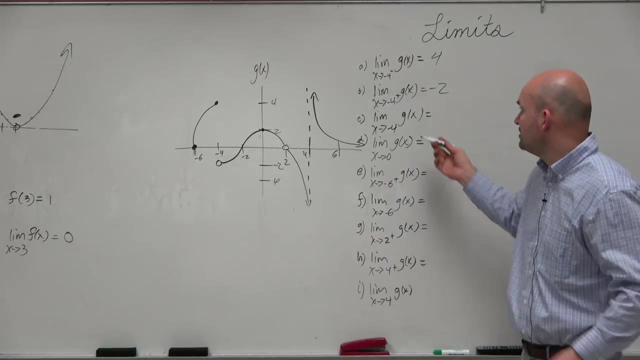 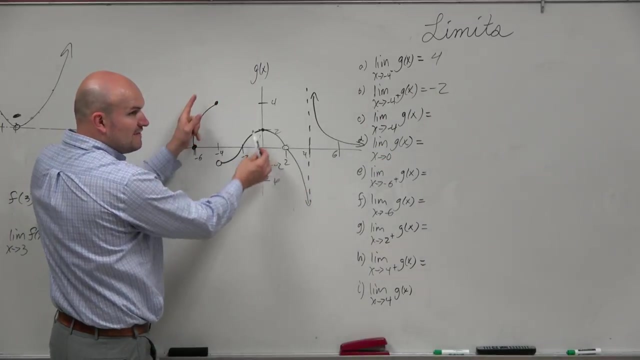 Now, this is helpful because if we want to identify what is our general limit, the general limit is the value that our function approaches from the left and from the right, And what we notice is, if I want to find the limit as x approaches negative 4, they don't approach the same value. 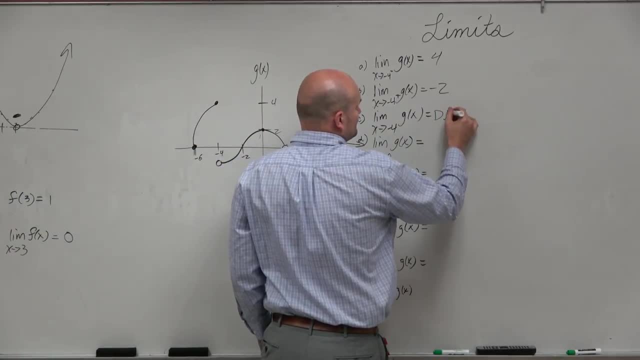 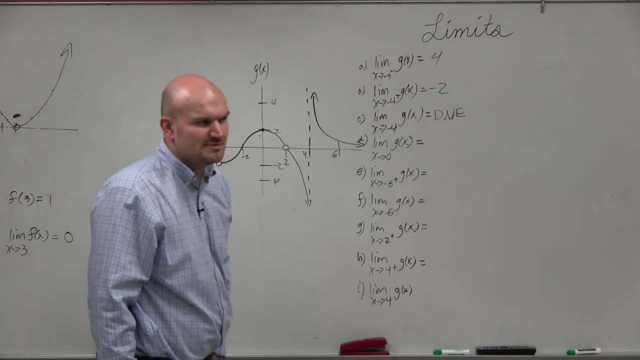 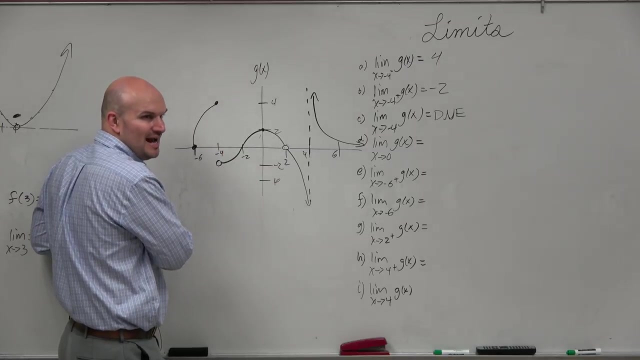 So guess what? The general limit does not exist. The limit as x approaches 0. Sometimes people are like: ah Well, guys, limits don't always have to occur at discontinuities. At x equals 0, we have the function is equal to 2.. 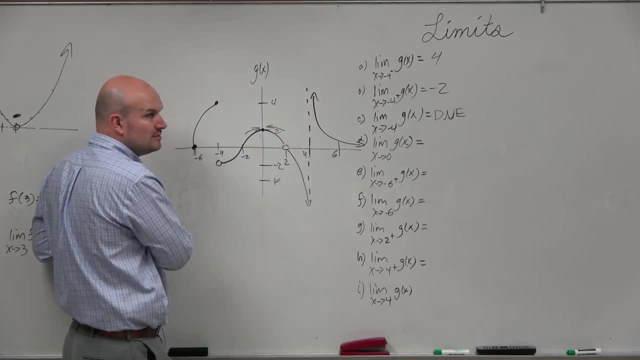 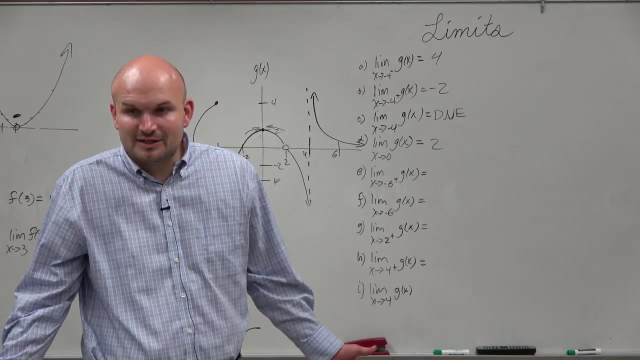 But as you guys see, as we approach from the left and through the right, what value are we approaching? 2. So it's a little gimme in there, But limits don't always have to approach at discontinuities. They're more likely to approach at discontinuities. 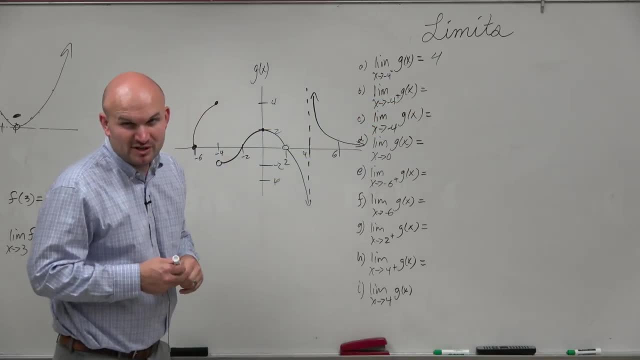 That little plus just means from the right hand side. So yeah, I would avoid just doing something that's not at least to your standard notation. So now let's go and take a look. What about, as we approach, negative 4 from the right? 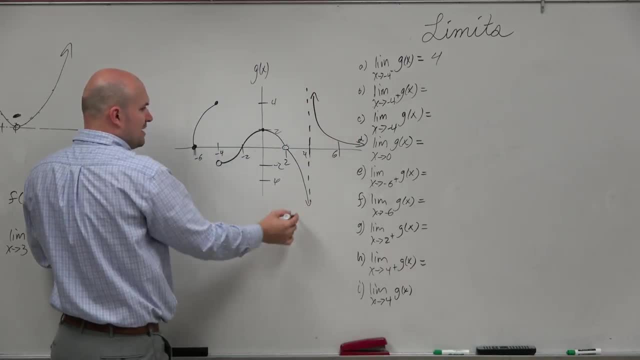 So we look at our graph, We kind of take out our right hand. We say, all right, let's follow this graph from the right. As we approach from the right, we get really, really close to which y value Negative 2.. 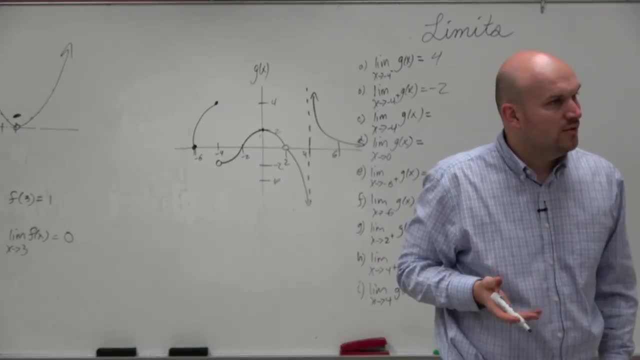 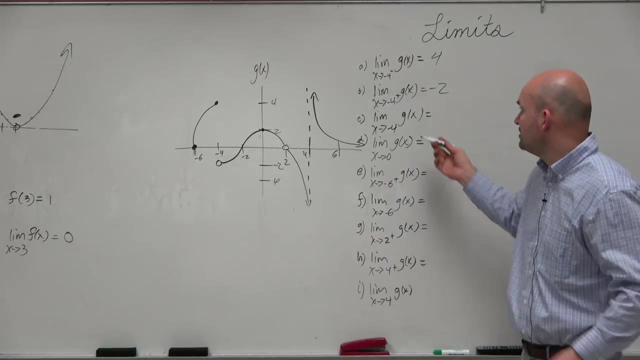 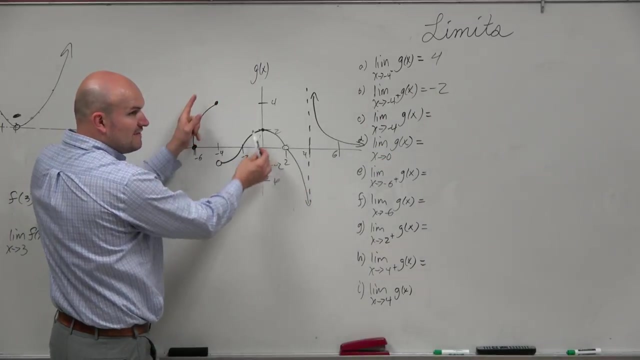 Now, this is helpful because if we want to identify what is our general limit, the general limit is the value that our function approaches from the left and from the right, And what we notice is, if I want to find the limit as x approaches negative 4, they don't approach the same value. 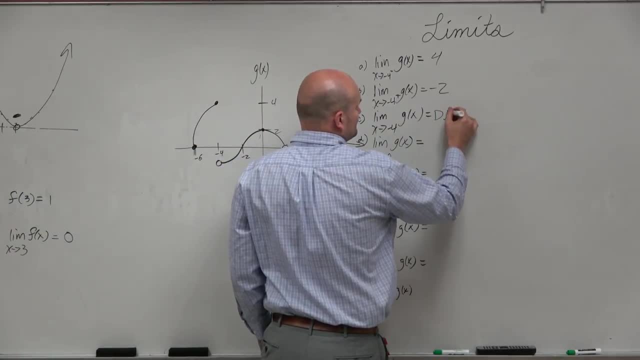 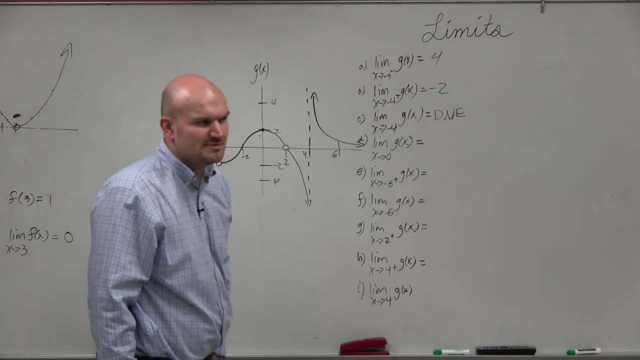 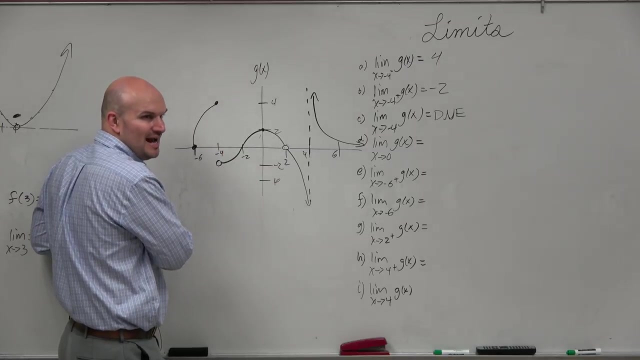 So guess what? The general limit does not exist. The limit as x approaches 0. Sometimes people are like: ah Well, guys, limits don't always have to occur at discontinuities. At x equals 0, we have the function is equal to 2.. 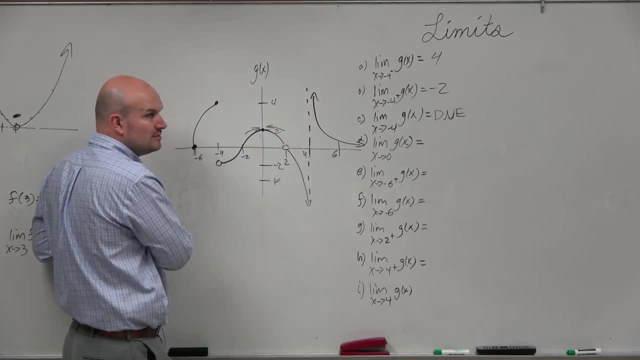 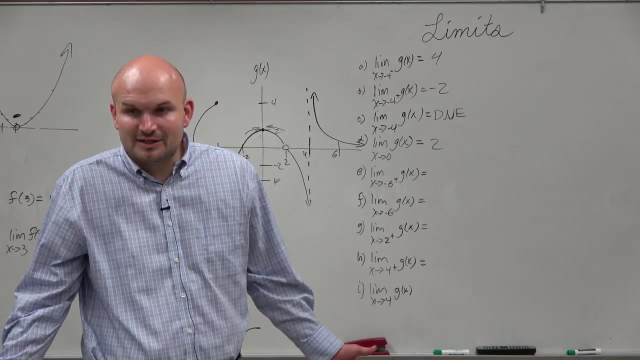 But as you guys see, as we approach from the left and through the right, what value are we approaching? 2. So it's a little gimme in there, But limits don't always have to approach at discontinuities. They're more likely to approach at discontinuities. 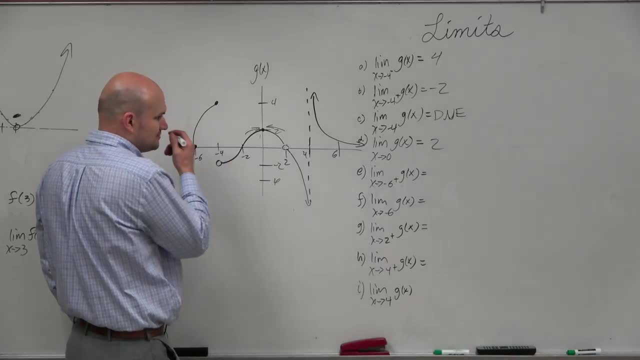 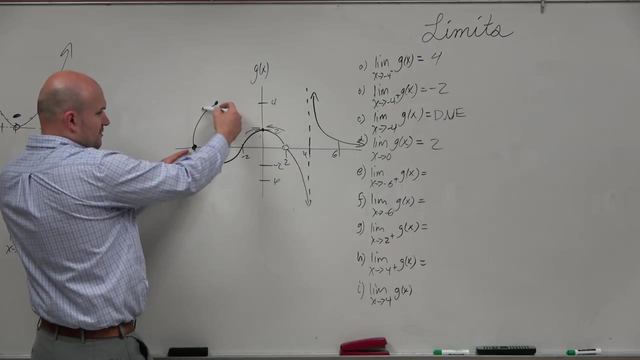 for algebraic reasons, which we'll see, But they don't always have to go to there. Next one: What about as we approach negative 6 from the right? So, as we're going from negative 6 from the right, we're getting really, really close to which y value? 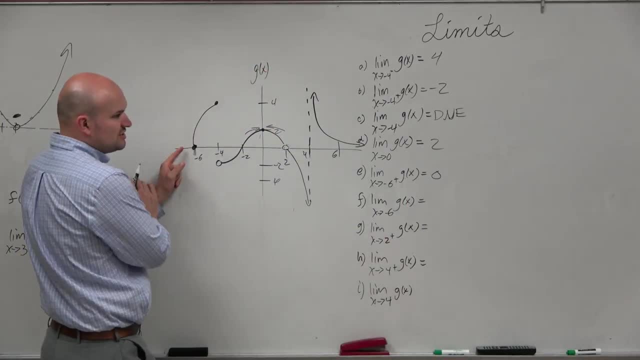 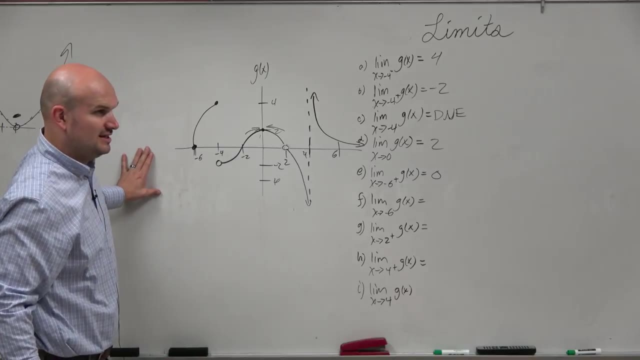 0.. What about as we approach the general limit from negative 6?? So, from the right, we're approaching 0.. From the left, is there anything on the left? No, No. So is it even possible to approach from the left? 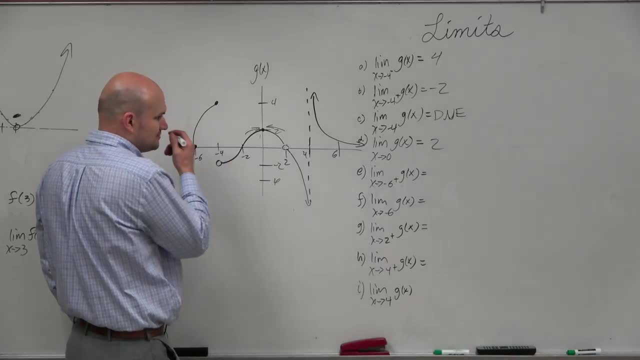 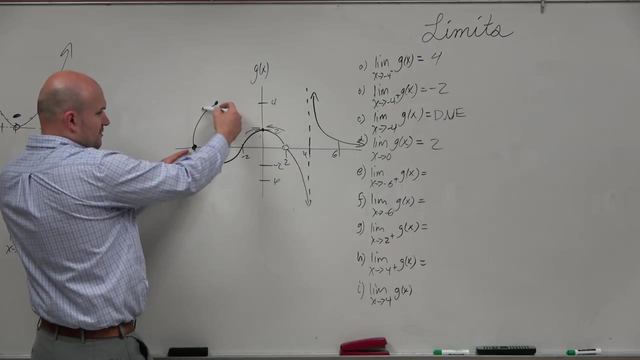 for algebraic reasons, which we'll see, But they don't always have to go to there. Next one: What about as we approach negative 6 from the right? So, as we're going from negative 6 from the right, we're getting really, really close to which y value? 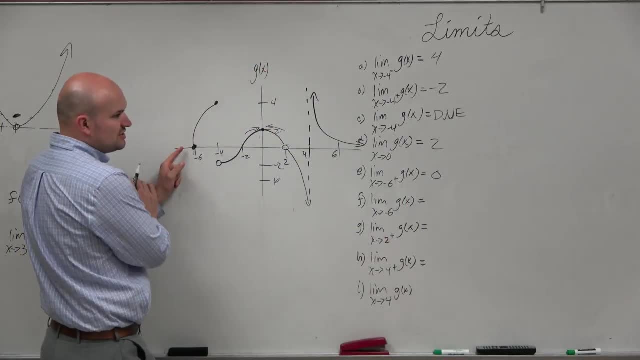 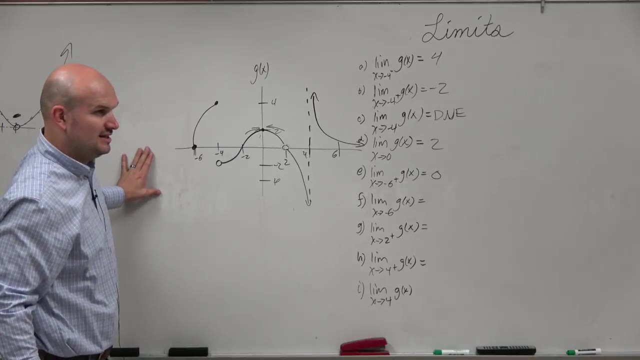 0.. What about as we approach the general limit from negative 6?? So, from the right, we're approaching 0.. From the left, is there anything on the left? No, No. So is it even possible to approach from the left? 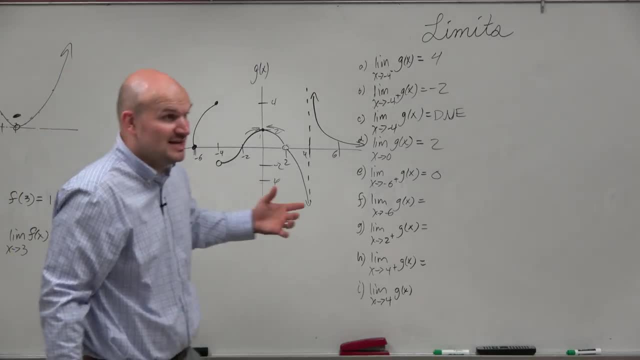 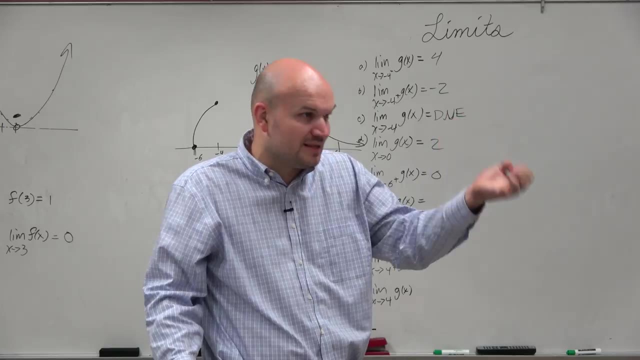 or there's nothing there, Not really. So since we don't have anything to the left, we can't approach from the left- right, And since our definition says we have to approach the same value from the left and the right, this does not exist. 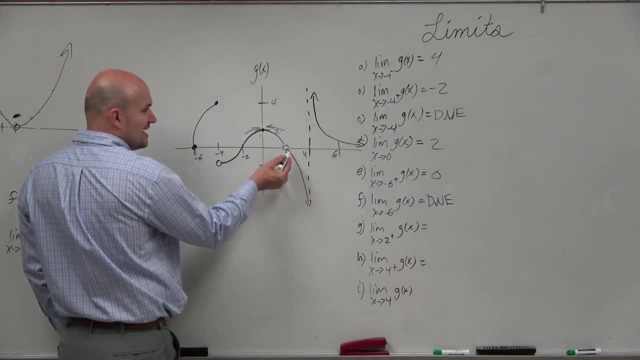 2 from the right. So, as we're approaching the value of 2 from the right, now again, here's a whole. But again, guys, it doesn't matter if it's a whole, It doesn't matter if there's a point there. 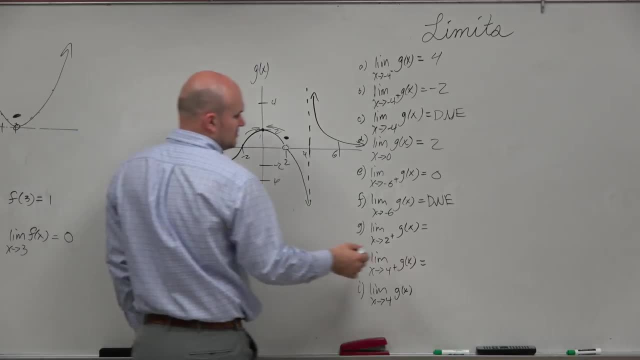 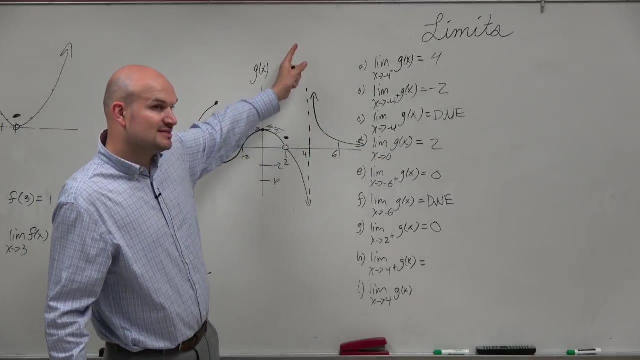 We're looking for the value which is approaching, which is 0. 0. 0.. As we approach 4, now this is an asymptote, right, But as we're approaching 4, from the right you guys can see that we're going all the way up to. 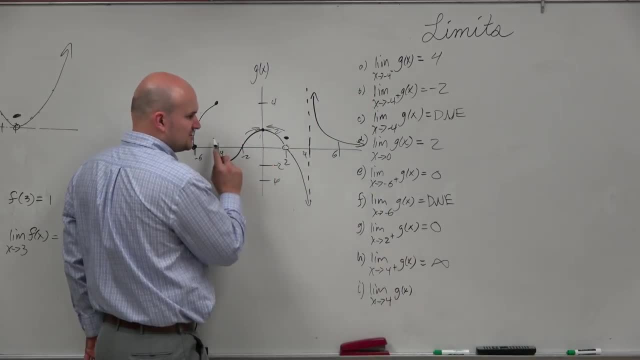 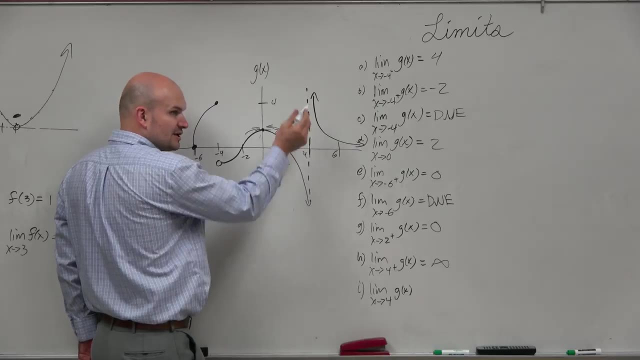 Infinity. And as we approach 4 from the left- or wait, this is just as we approach 4 from the left- we're going down to negative 50.. Well, since we're not approaching the same, since we're going in different directions here at 4,. 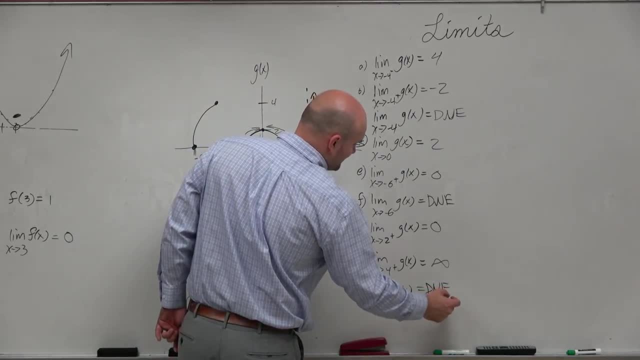 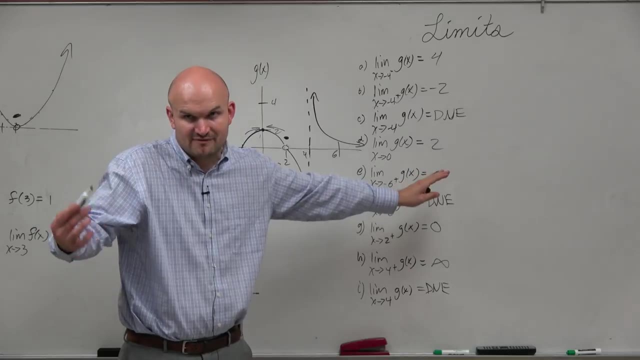 we can definitely say it does not exist. Now technically, real quick, technically from 4 from the right, still does not exist because you're not actually approaching a y value. infinity is not a value, But a lot of times we give the direction. 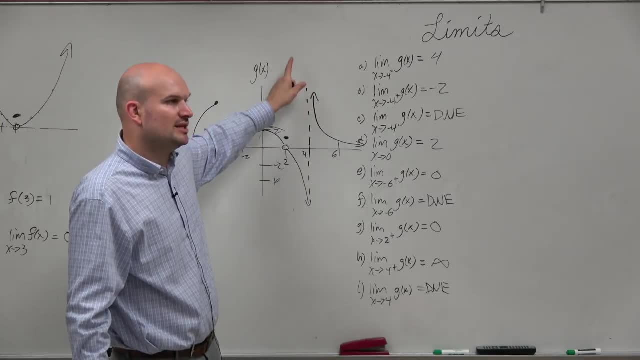 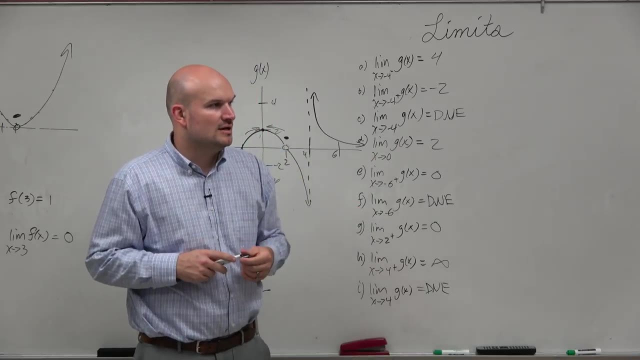 that the graph is heading. when we're approaching an asymptote or n behavior or something like that, We give the direction because the direction is more specific than does not exist. But technically, 4 positive does not exist because you're actually not approaching a value. 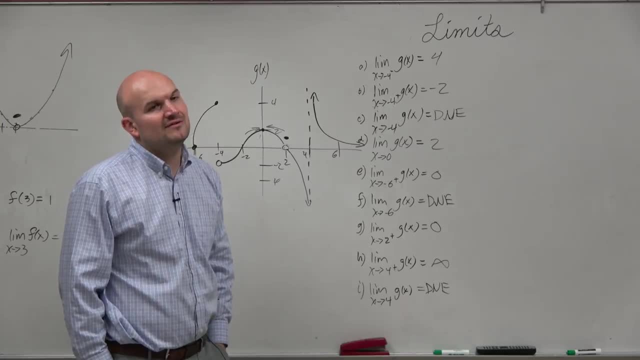 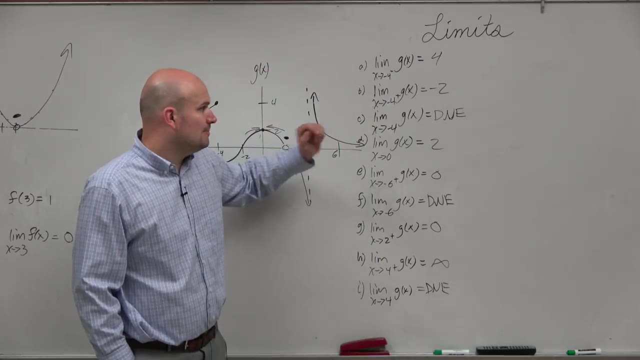 Yes, What if we get that question? You wouldn't have to choose between does not exist and infinity No, So that's what I'm just saying. Like technically it does not exist, But we often- rather you- just label the direction. 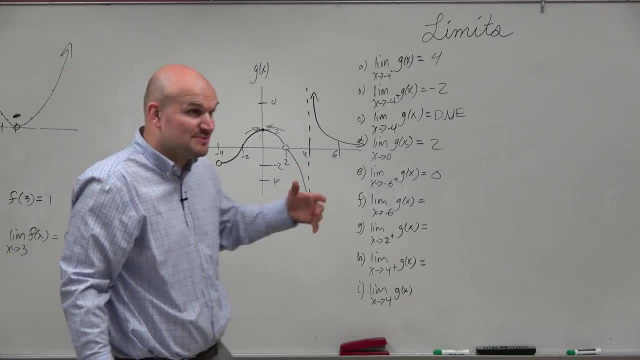 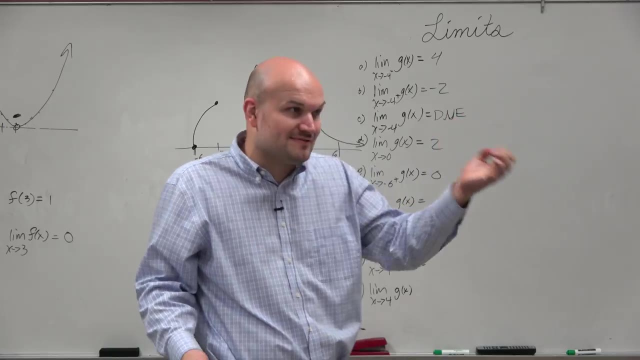 or there's nothing there, Not really. So since we don't have anything to the left, we can't approach from the left- right, And since our definition says we have to approach the same value from the left and the right, this does not exist. 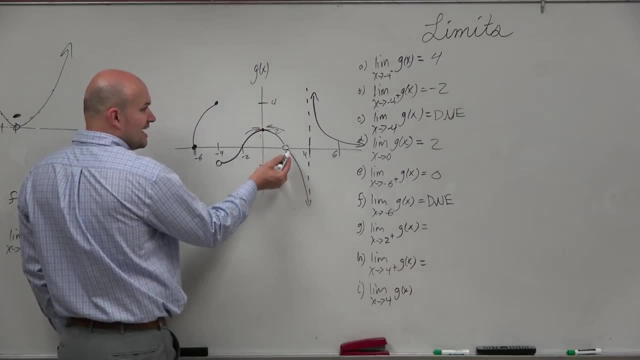 2 from the right. So, as we're approaching the value of 2 from the right, now again, here's a whole. But again, guys, it doesn't matter if it's a whole, It doesn't matter if there's a point there.